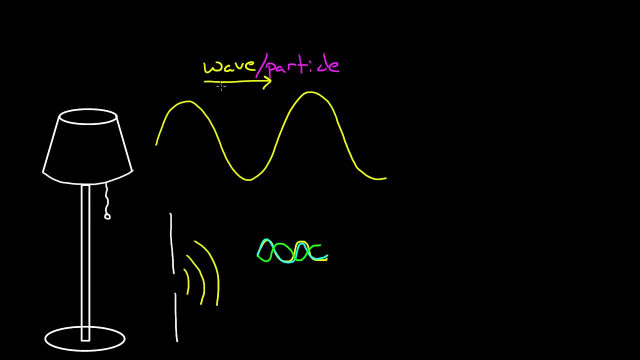 localized in some region of space. waves can get localized. if you sent in some wave here, that was a wave pulse. well, that wave pulse is pretty much localized. when it's traveling through here it's going to kind of look like a particle. that's not really what we mean. we mean something more dramatic. we mean that light. what physicists discovered is that light and light particles can only deposit certain amounts of energy. 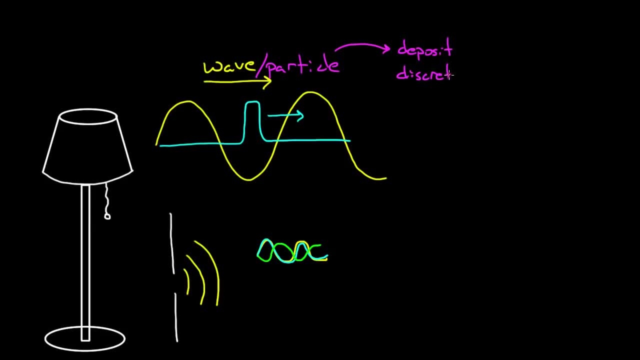 only discreet amounts of energy. there's a certain chunk of energy that light can deposit, no less than that. so this is why it's called quantum mechanics. you've heard of a quantum leap. quantum mechanics means a discreet jump, no less than that. and so what do we call these particles of light? we call them photons. how do we draw them? that's a little trickier, we know now. 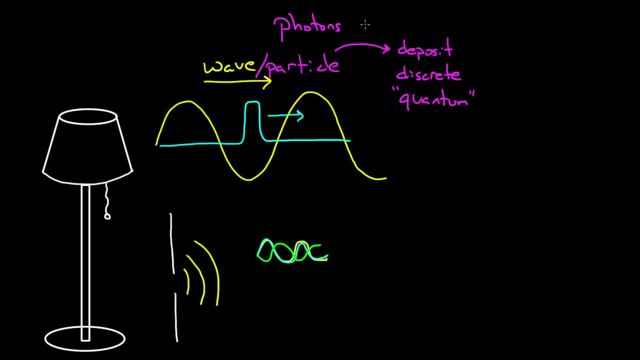 Light can behave like a wave and a particle, so we kind of split the difference sometimes. Sometimes you'll see it like this, where it's kind of like a wavy particle: So there's a photon, here's another photon. Basically, this is the problem. 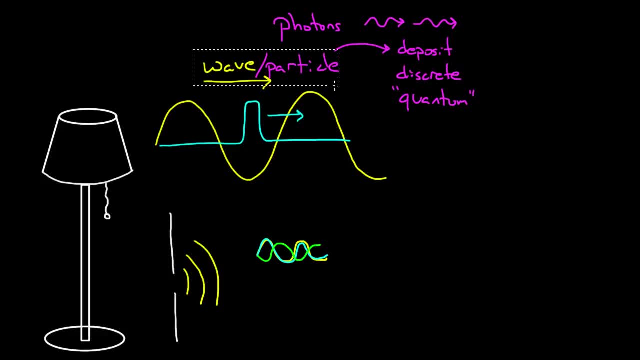 This is the main problem with wave-particle duality. it's called the fact that light, and everything else for that matter, can behave in a way that shows wave-like characteristics. It can show particle-like characteristics. There's no classical analog of this. 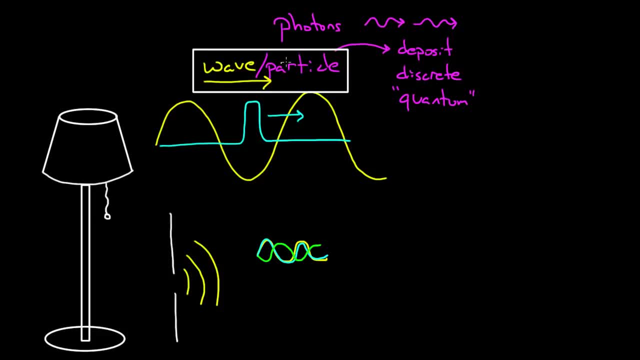 We can't envision in our minds anything that we've ever seen that can do this, that could both behave like a wave and a particle. So it's impossible basically to draw some sort of visual representation, but it's always good to draw something. 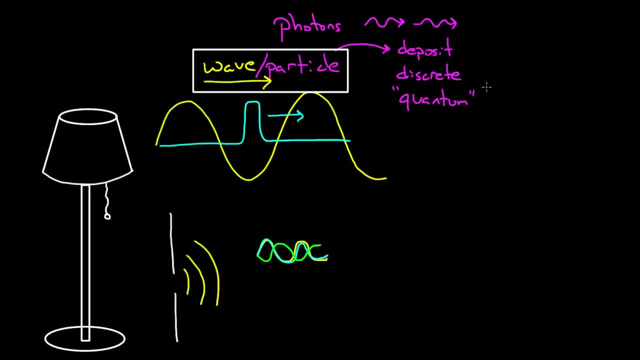 So we draw our photons like this, And so what I'm really saying here is if you had a detector sitting over here that could measure the light energy that it receives from some source of light, what I'm saying is that if that detector was sensitive enough, 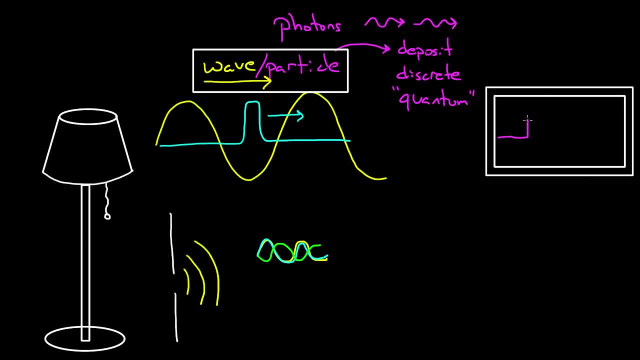 you'd either get no light energy or one jump, or no light energy or whoop. you absorbed another photon. You couldn't get in between. If the quantum jump was three units of energy. I don't wanna give you a specific unit yet. 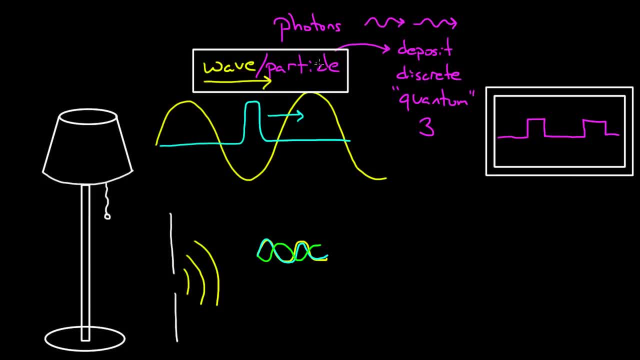 but say three units of energy you could absorb if that was the amount of energy for that photon. if these photons were carrying three units of energy, you could either absorb no energy whatsoever or you could absorb all three. You can't absorb half of it. 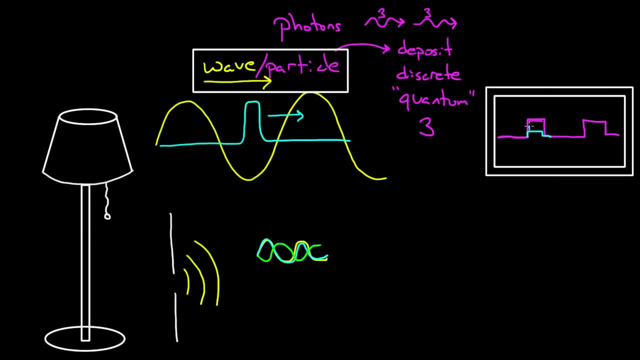 You can't absorb one unit of energy or two units of energy. You could either absorb the whole thing or nothing. That's why it's quantum mechanics. You get this discrete behavior of light, depositing all its energy in a particle-like way or nothing at all. 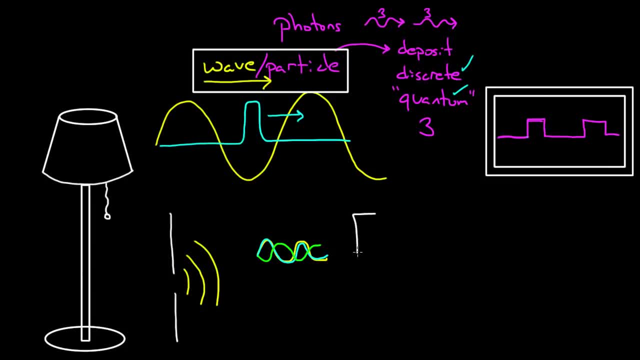 How much energy? Well, we've got a formula for that. The amount of energy in one photon. It's determined by this formula. The first thing in it is Planck's constant. H is the letter we use for Planck's constant. 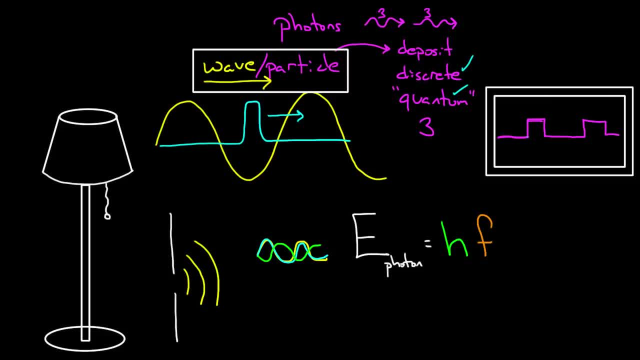 and times F. this is it. It's a simple formula. F is the frequency. What is Planck's constant? Well, Planck. Planck was basically the father of quantum mechanics. Planck was the first one to figure out what this constant was and to propose. 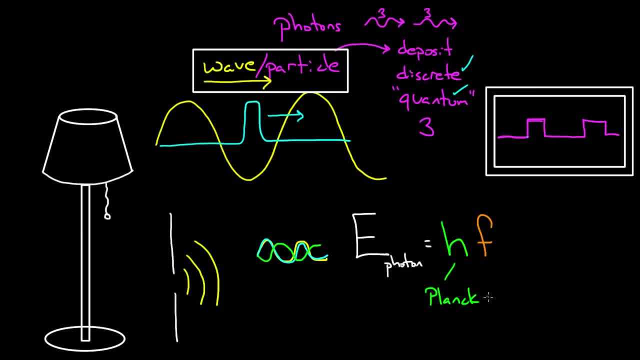 that light can only deposit its energy in discrete amounts. So Planck's constant. it is extremely small. It's 6.626 times 10 to the negative 34th. joule times: seconds: 10 to the negative 34th. 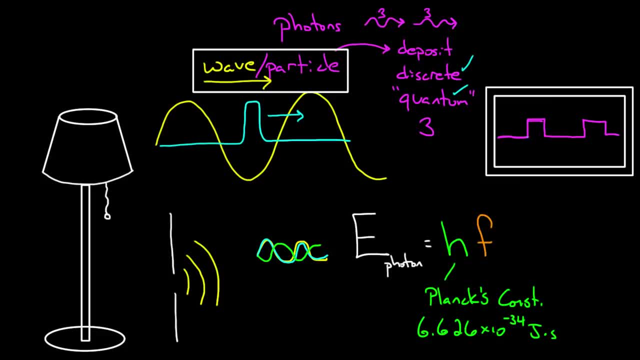 There aren't many other numbers in physics that small Times the frequency. This is regular frequency. So frequency: number of oscillations per second measured in hertz. So now we can try to figure out. why did physicists never know and never discover this before? 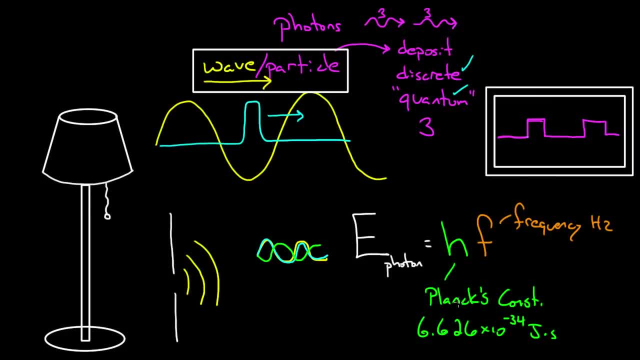 And the reason is Planck's constant is so small that the energy of these photons are extremely small. The graininess of this discrete amount of energy that's getting deposited is so small that it just looks smooth. You can't tell that there's a smallest amount. 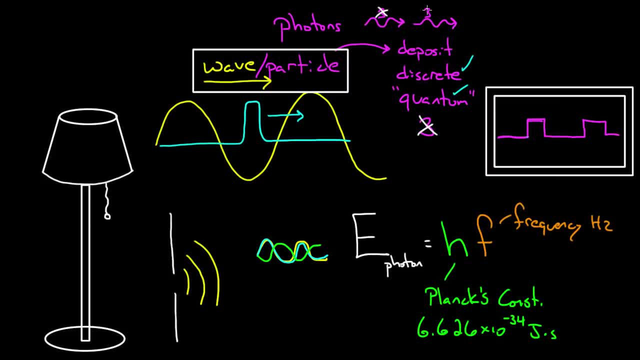 or at least it's very hard to tell. So instead of just saying three units, let's get specific for violet light. So you had a violet. what's the? what's the, what's the energy of one violet photon? 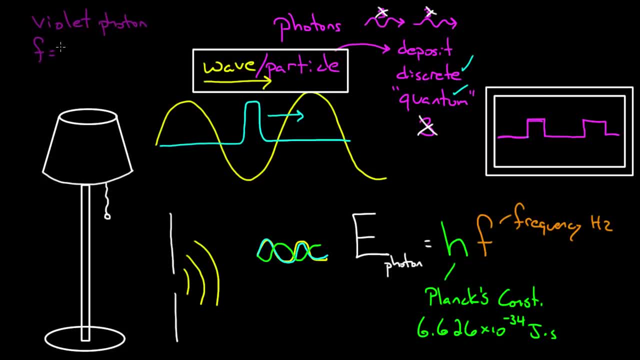 Well, the frequency of violet light is 7.5 times 10 to the 14th hertz. So if you take that number times this Planck's constant, 6.626 times 10 to the negative 34th, 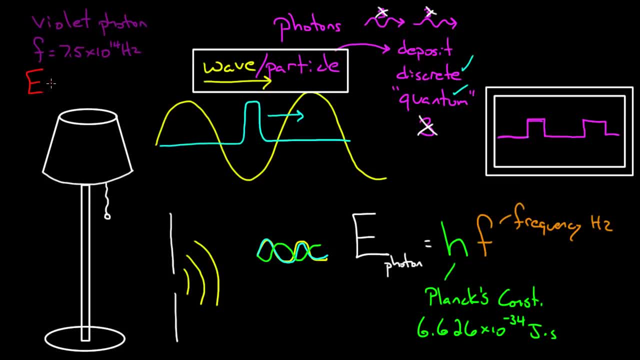 you'll get that the energy of one violet photon is about 5 times 10 to the negative 19th Joules. 5 times 10 to the negative 19th. that's extremely small. that's hard to see, that's hard to notice that energy's coming. 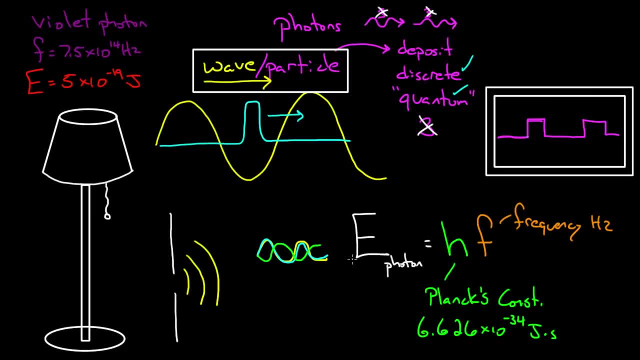 in this discrete amount. It's like water. I mean water from your sink. Water flowing out of your sink looks continuous. We know there's really discrete water molecules in there and that you can only get one water molecule. no water molecules. 10 water molecules. 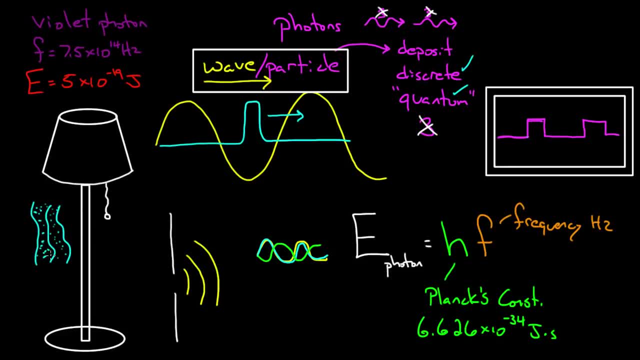 discrete amounts of these water molecules, but there's so many of them and they're so small. it's hard to tell that it's not just completely continuous. The same is happening with this light. This energy's extremely small. Each violet photon has an extremely small amount of energy. 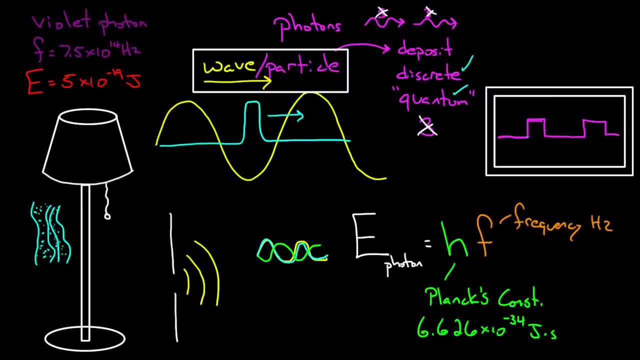 that it contributes. In fact, if you wanted to know how small it is- a baseball, a professional baseball player throwing a ball fast- you know it's about 100 joules of energy. If you wanted to know how many of these photons. 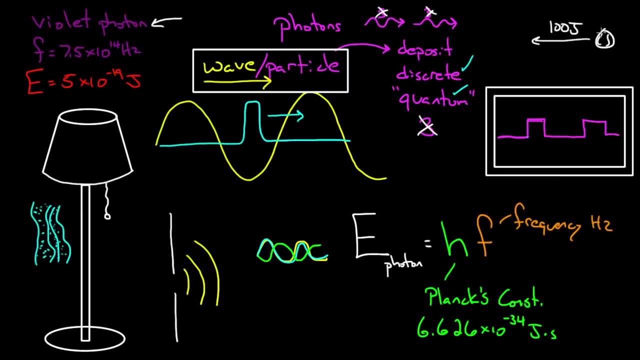 how many of these violet photons would it take to equal the energy of one baseball thrown at major league speed? it would take about 2 million trillion of these photons to equal the energy in a baseball that's thrown. That's why we don't see this on a macroscopic scale. 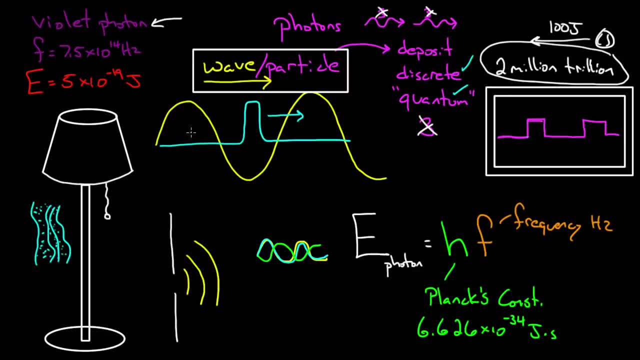 For all intents and purposes, for all we care. at a macroscopic level light's basically continuous. It can deposit any energy whatsoever Because the scale's so small here. But if you look at it up close, light can only deposit discrete amounts. 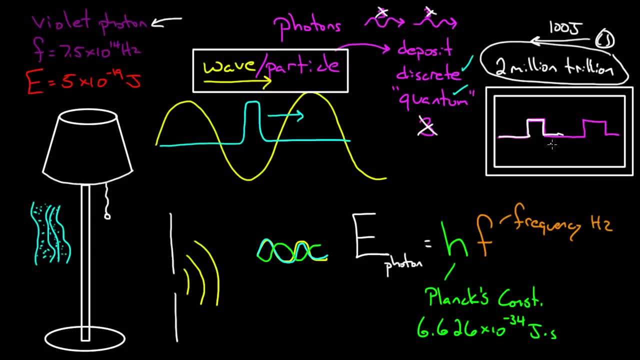 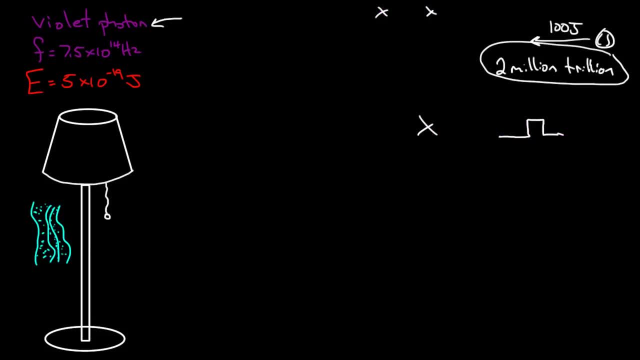 Now I don't mean that light can only deposit small amounts. Light can deposit an enormous amount of energy, but it does so in chunks. So think about it this way. Let's get rid of all this. Think about it this way. Let's say you had a detector that's gonna register.